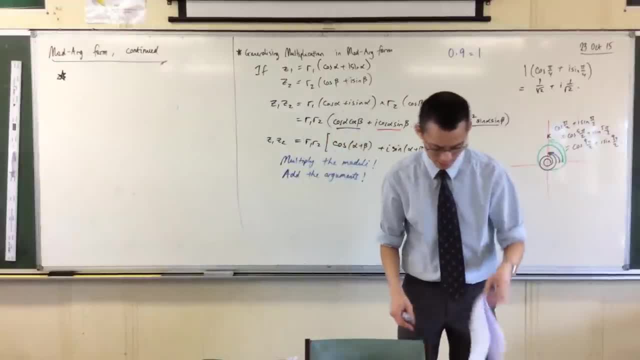 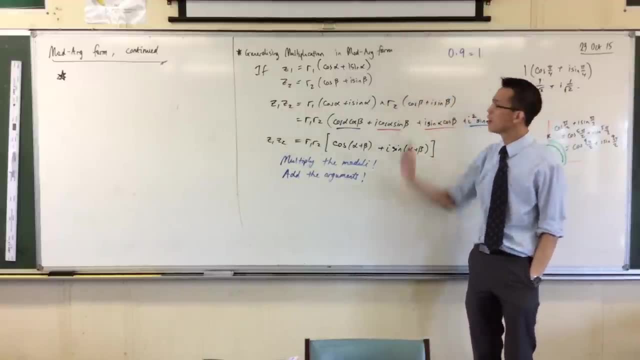 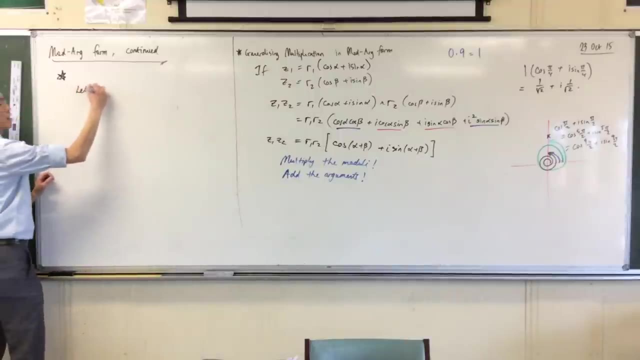 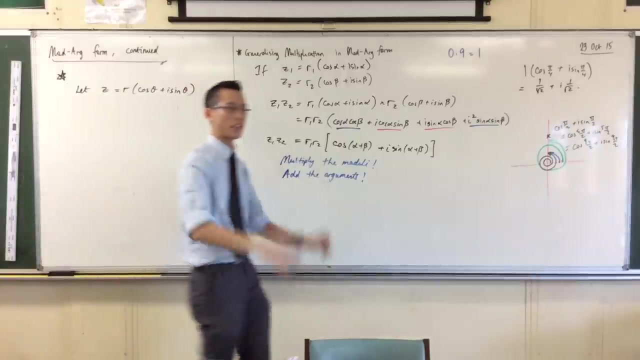 What I want you to think about here is the particular case where I don't multiply by. I don't multiply two different complex numbers, but what if I multiply the same complex number repeatedly? okay, So let's, let's just come up with this guy: r cos theta plus i sin theta. So here's your generic complex number in mod r form. okay. 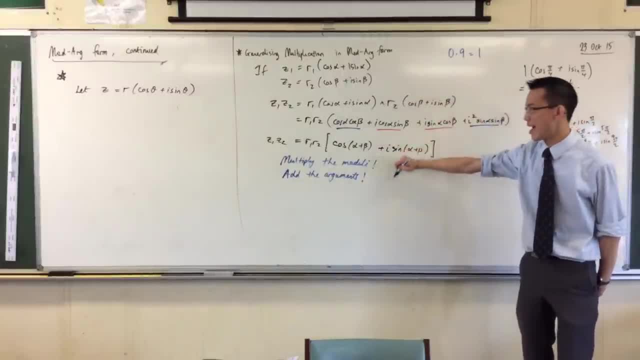 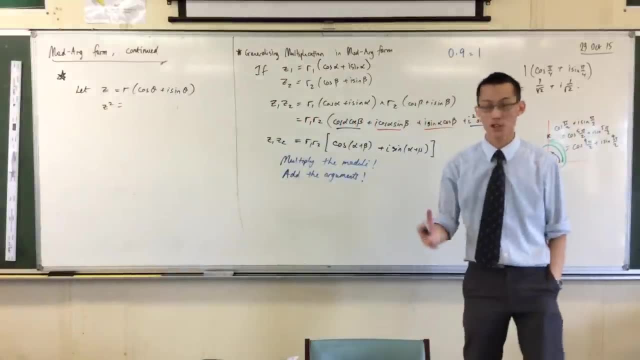 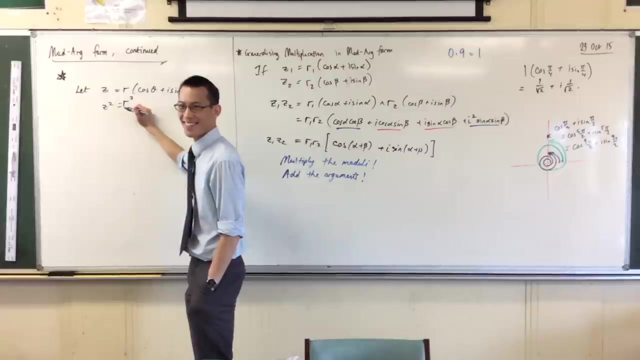 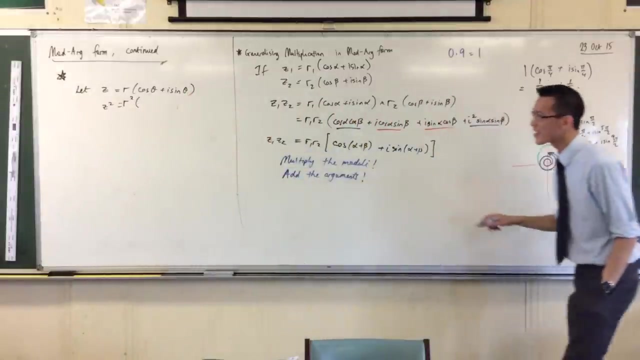 Using this principle of multiplying the moduli and adding the arguments. okay, What's z squared First, we'll do the moduli. Yeah, Vincey, R squared. I'm laughing, though. This is the third question. the second question that none of us can get: 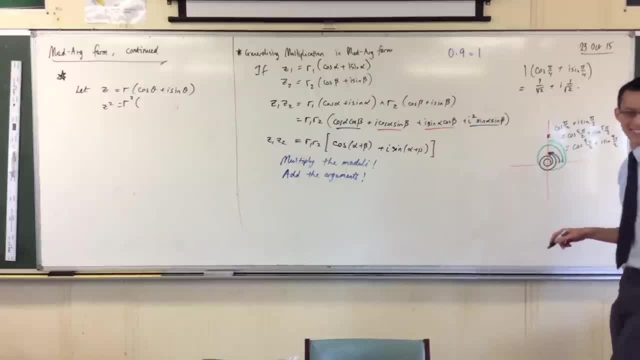 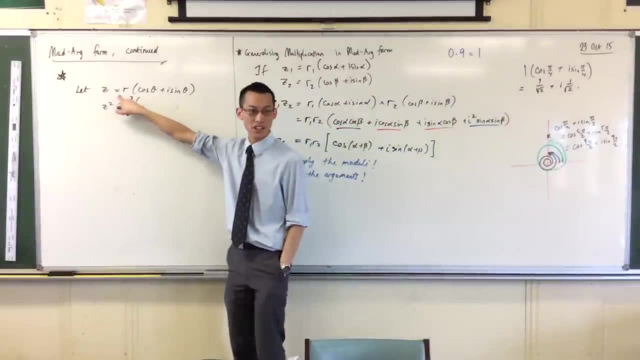 I'm not finished yet. I'd like to: Don't, don't, don't, don't. go too hard on yourself, okay, Alright, hold on a sec. I've multiplied the moduli right: R times r. Now I add the arguments: right. 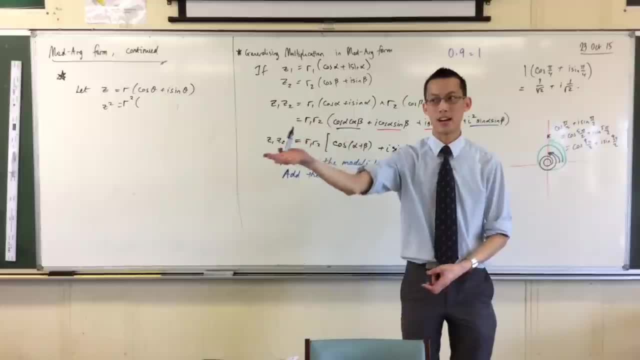 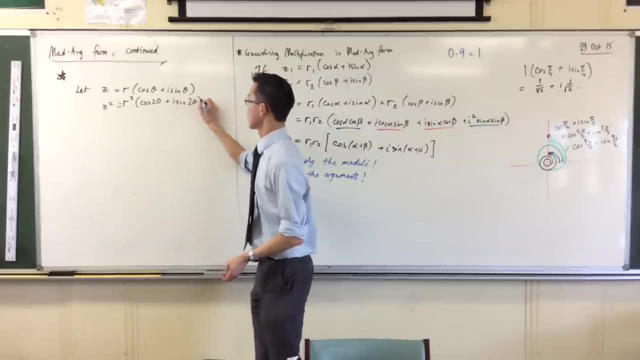 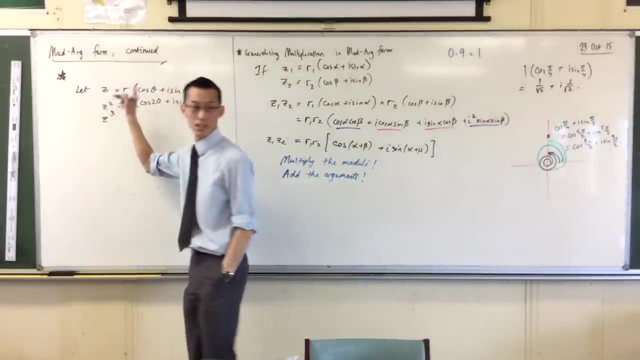 Now if I'm adding the argument to itself, theta plus theta, it's just going to be cos 2 theta plus i sin 2 theta. Okay with that. Now what if I did it again? okay If I multiply by z the original one another time: okay. 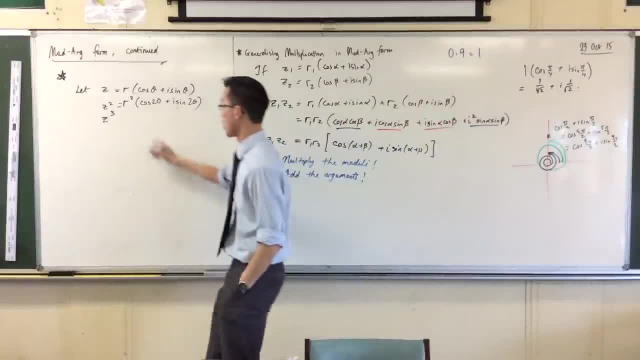 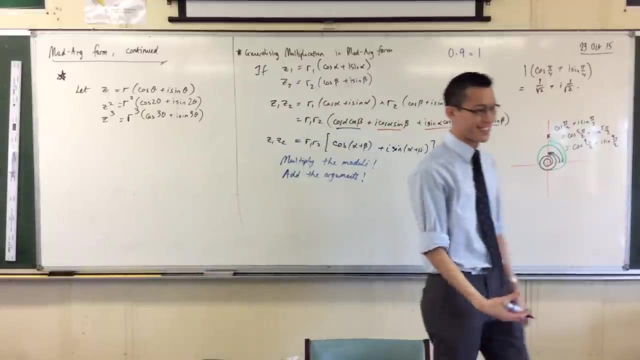 Will I multiply by the same modulus, So I get r cubed And then I add the same argument, which is still theta, right? So this guy's going to be cos 3 theta plus i sin 3 theta. okay, Now it doesn't take a rocket scientist to generalize from here, right? 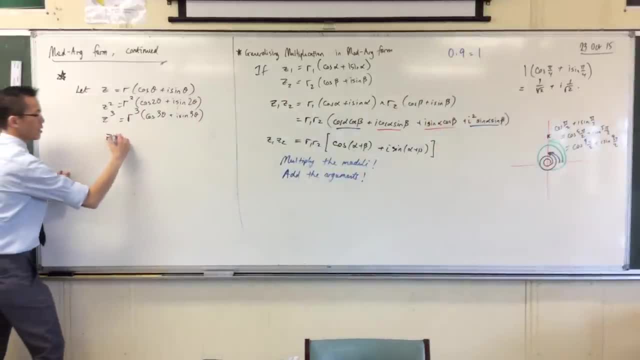 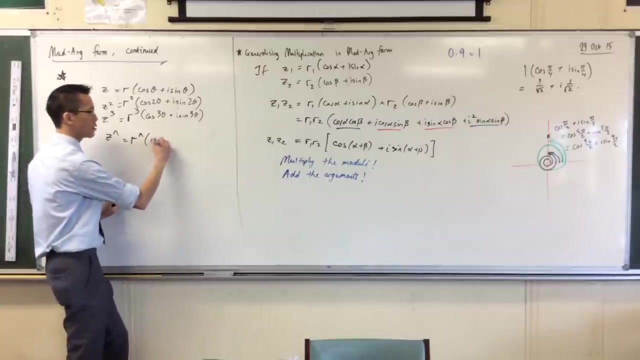 If you take any complex number and you raise it to some integer power, okay, I'm going to write down my condition, my restriction, in a second. If I raise it to an integer power, then all I need to do is raise the modulus to that same integer power and multiply my angle by whatever power it was okay. 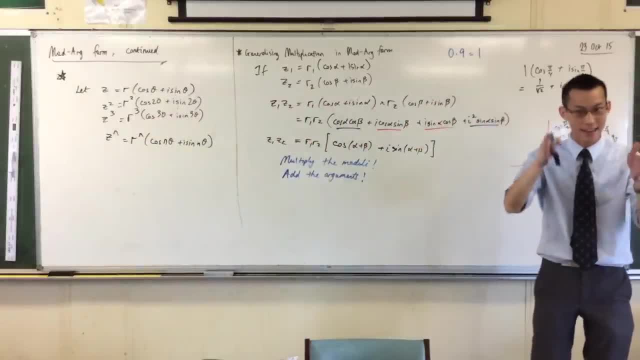 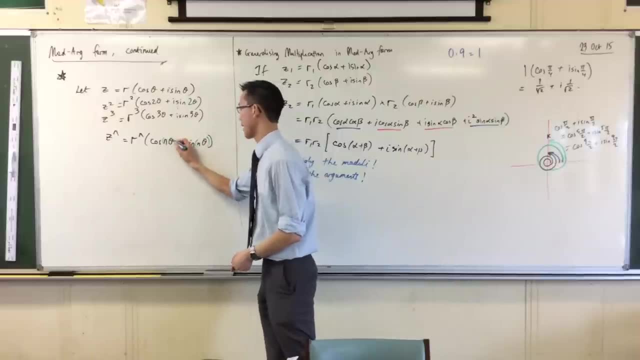 Now don't read out. it's not a double n, That's i sin n theta And sometimes, to make that really obvious, some mathematicians and authors and textbooks will put brackets around there, just to make it really really obvious. Okay. 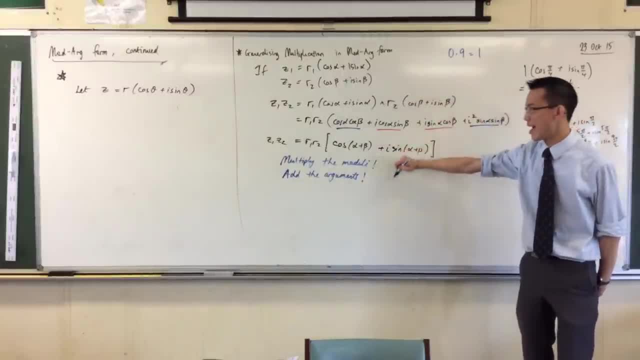 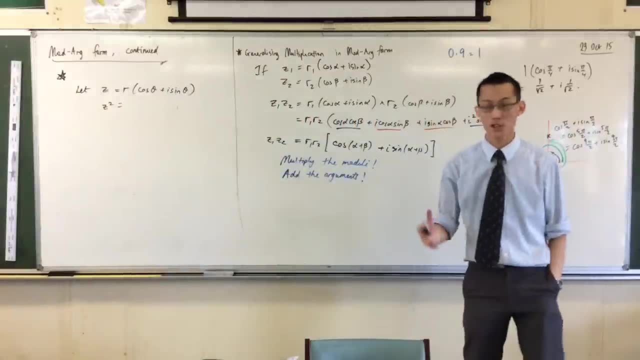 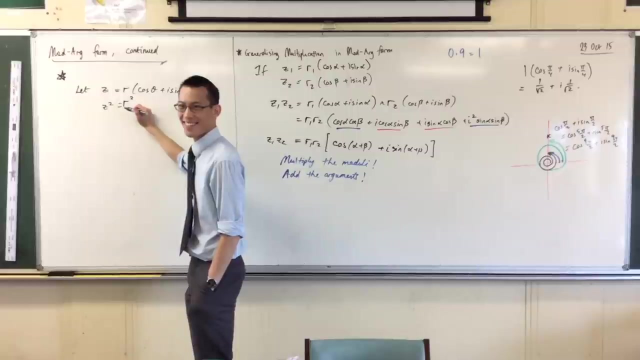 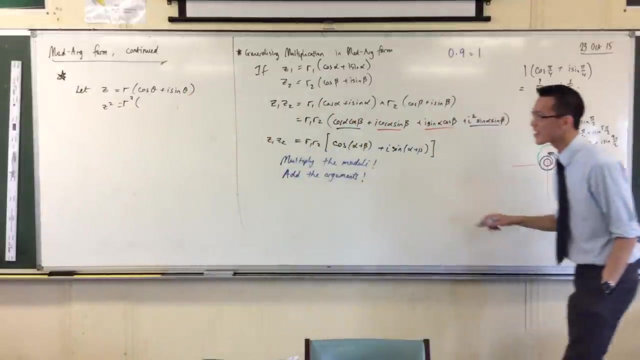 Using this principle of multiplying the moduli and adding the arguments. okay, What's z squared First, we'll do the moduli. Yeah, Vincey, R squared You? alright, What? I'm laughing, I don't know. This is the third question. the second question that no one, none of us, can get: 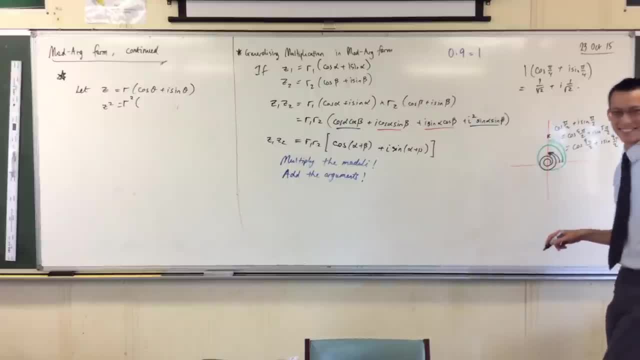 I'm not finished yet, I'd like to. I'm not finished yet, I'd like to, I'd like to. Don't, don't, don't, Don't go too hard on yourself, okay, Alright, hold on a sec. 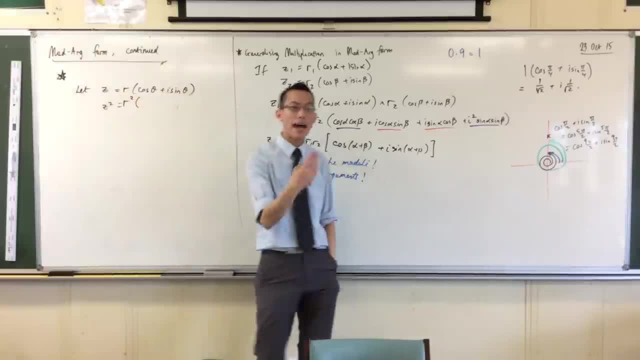 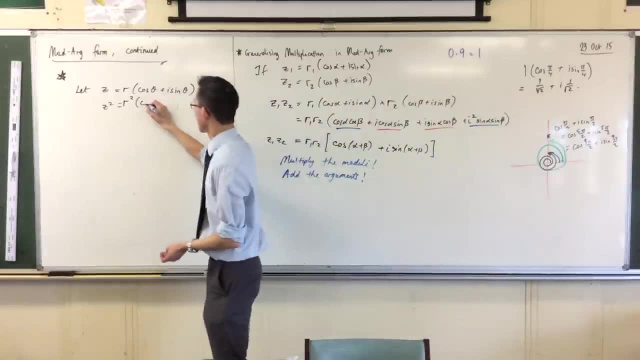 I've multiplied the moduli right R times r. Now I add the arguments right Now. if I'm adding the argument to itself, theta plus theta, it's just going to be cos 2 theta plus i sin 2 theta. 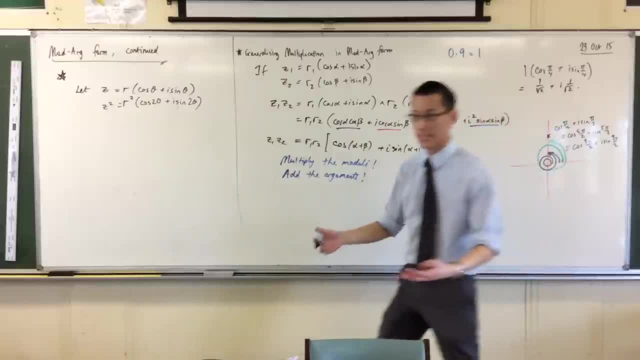 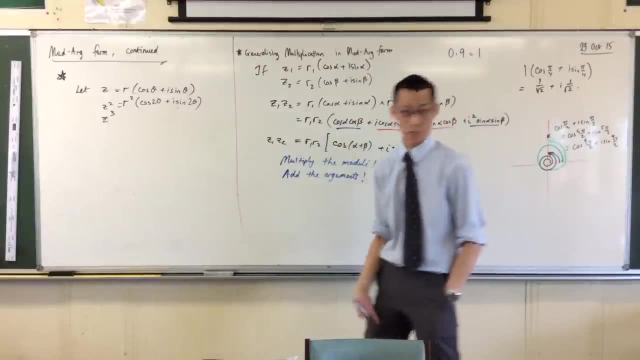 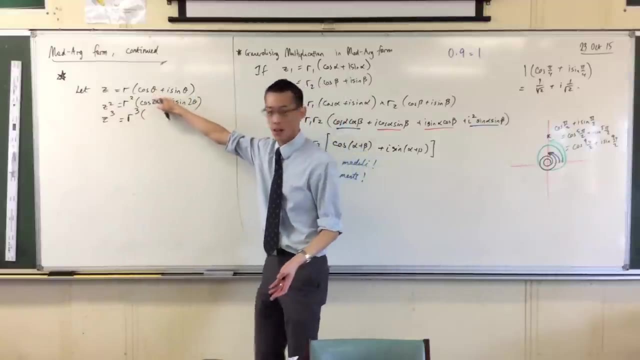 Okay with that. Now what if I did it again? Okay, if I multiply by z the original one another time. okay, Will I multiply by the same modulus, So I get r cubed, and then I add the same argument, which is still theta right. 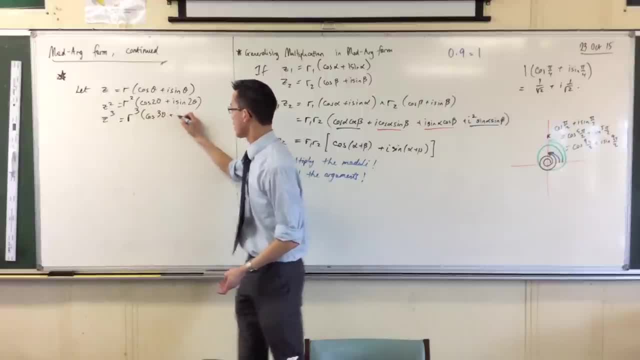 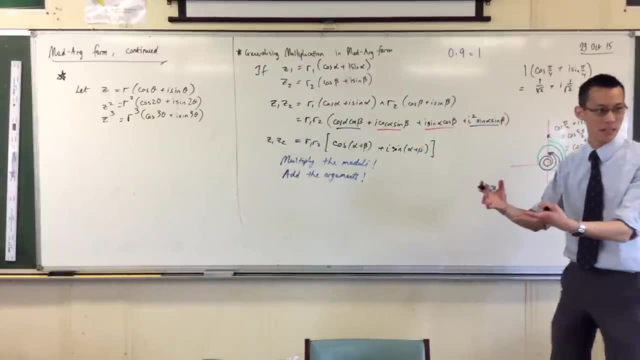 So this guy's going to be cos 3 theta plus i sin 3 theta. okay, Now it doesn't take a rocket scientist to generalize from here, right, If you take any complex number and you raise it to some integer power. okay. 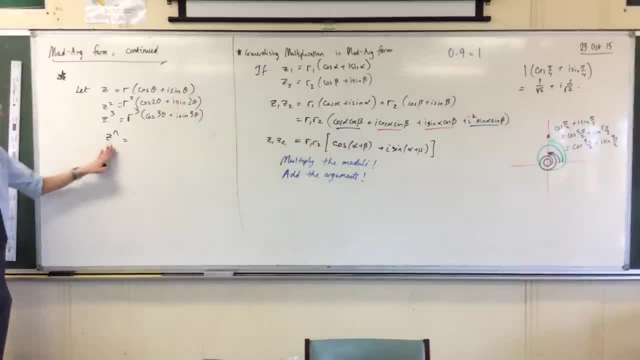 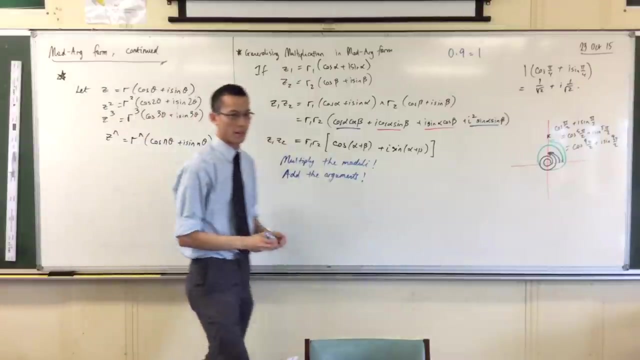 I'm going to write down my condition, my restriction, in a second. If I raise it to an integer power, then all I need to do is raise the modulus to that same integer power and multiply my angle by whatever power it was Okay. 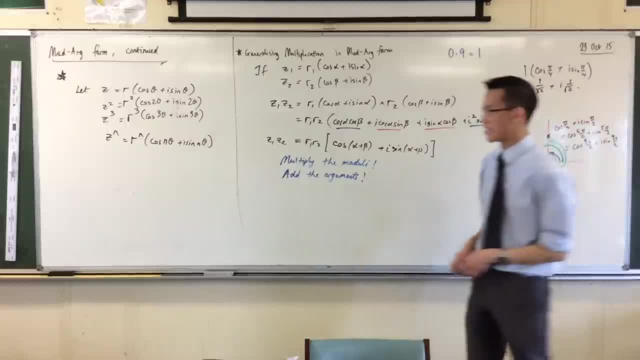 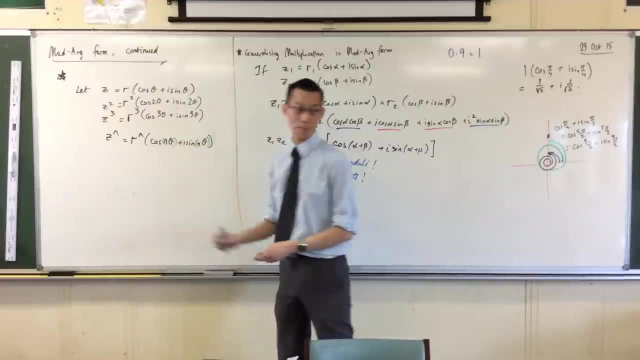 Now don't read out. it's not a double n, That's i sin n theta And sometimes, to make that really obvious, some mathematicians and authors and textbooks will put brackets around there, just to make it really really obvious. Okay. 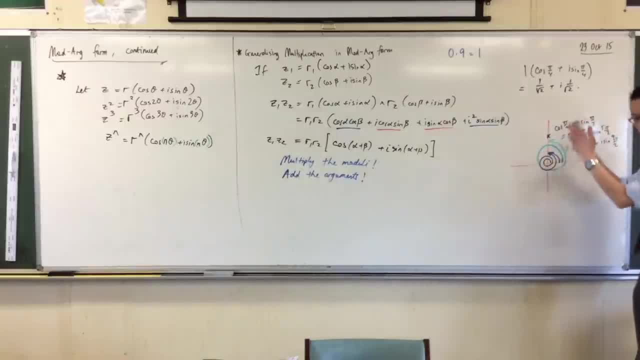 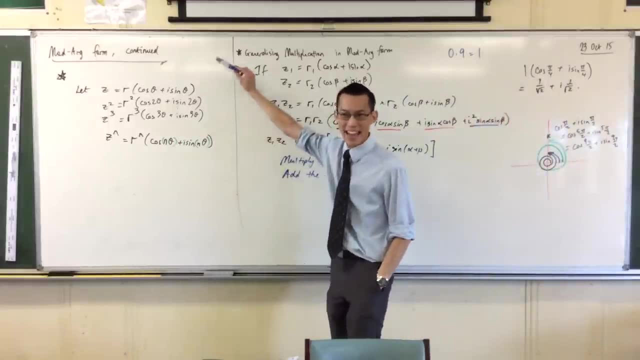 Now, you remember I said The complex plane. right, We call it the Argand diagram. Argand was a French mathematician. Another French mathematician came up with this. Now, this is the name I'm going to put on this, okay. 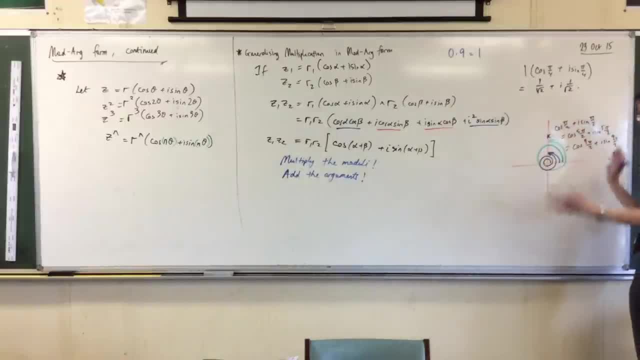 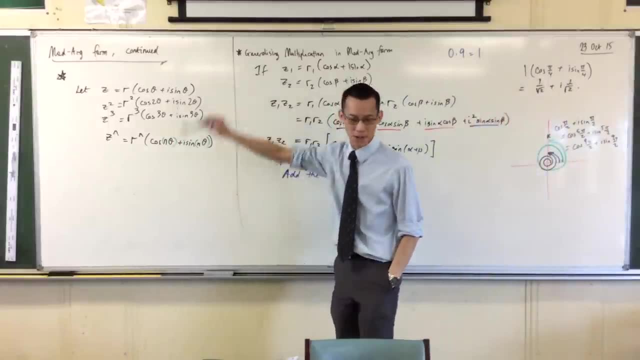 So remember, I said the complex plane, right, We call it the Argand diagram. Argand was a French mathematician. Another French mathematician came up with this. Now, this is the name I'm going to put on this, okay, And I'm going to write it first, and then I'm going to teach you how to pronounce it, okay. 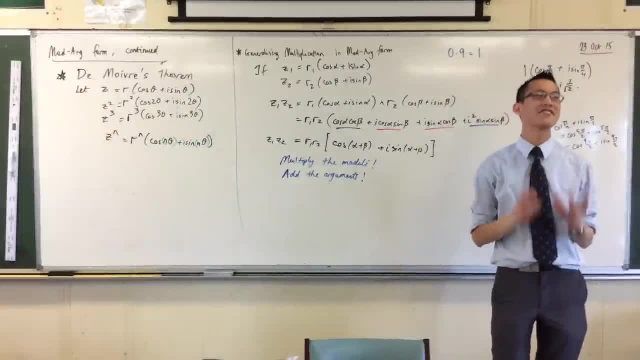 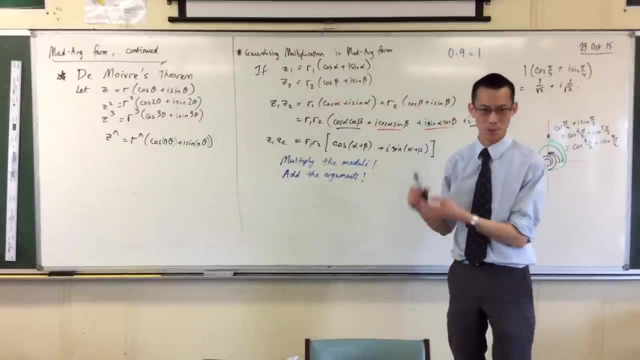 So here is the theorem. Now I have heard like a hundred different pronunciations of this name. okay, Let me teach you first, like the pieces, before we do this thing. okay, Firstly, remember, It's French, right, It's French. 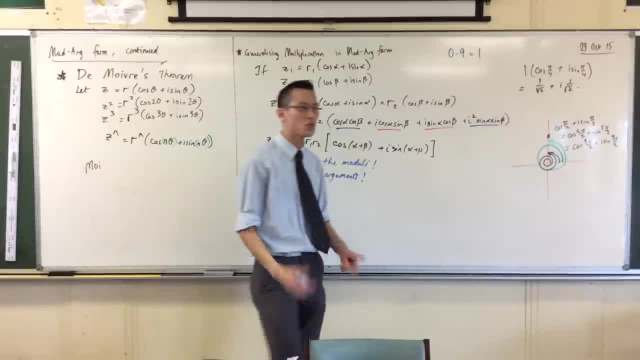 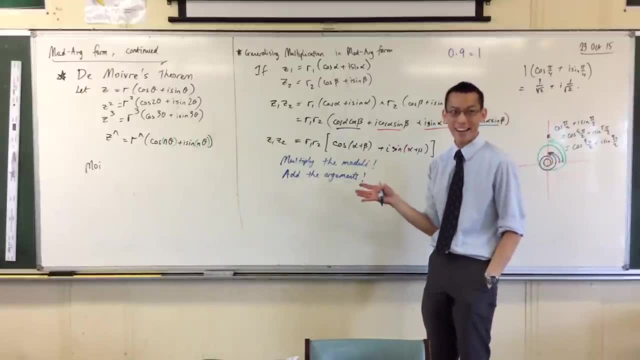 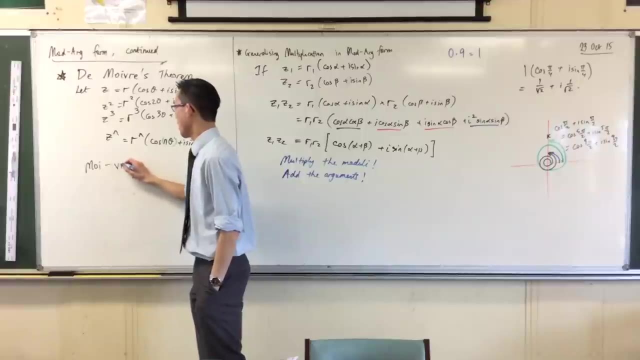 So in French, when you see this word, what do you say? You say moi right, As in you know me, okay. You do not say moi okay, Don't say moi Now. secondly, when you see this: okay. 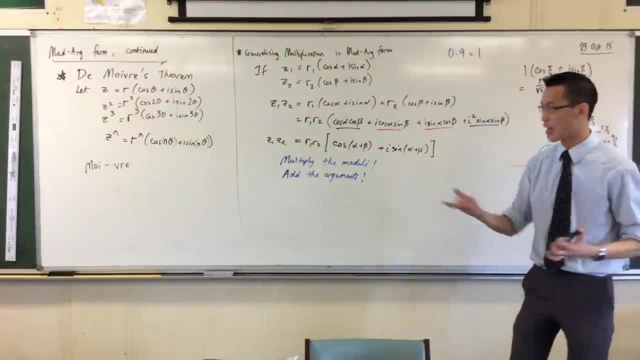 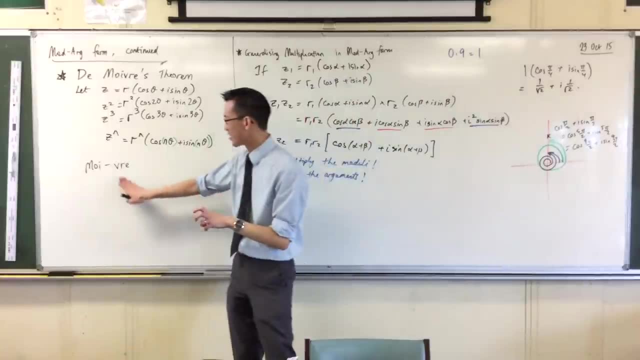 Now you might know, there's a famous art gallery which has this as the end of its name as well. okay, Now it's this R here, right, It's not quite like we say R. There's no vowel in here, okay. 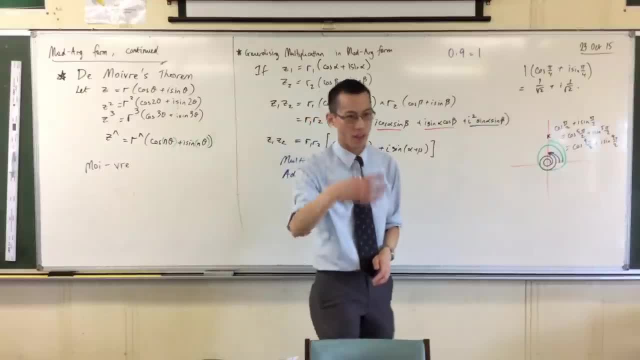 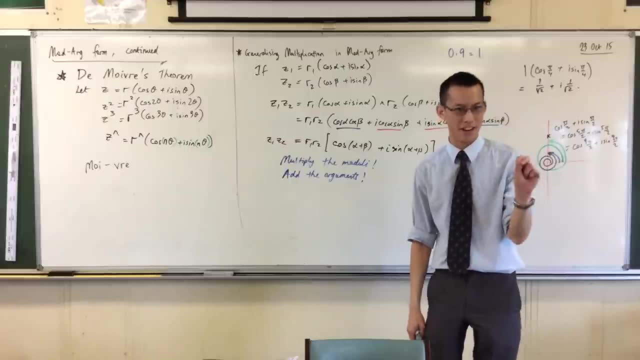 So the way you would say this is: as It's not like There's no hard R sound on the end, It's just You almost don't hear it. okay, You almost don't hear it. This is de Moivre's theorem, okay. 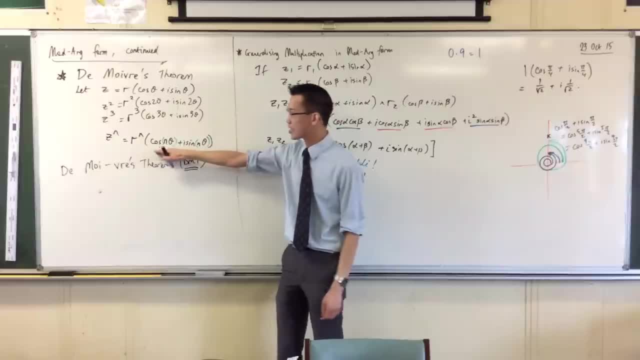 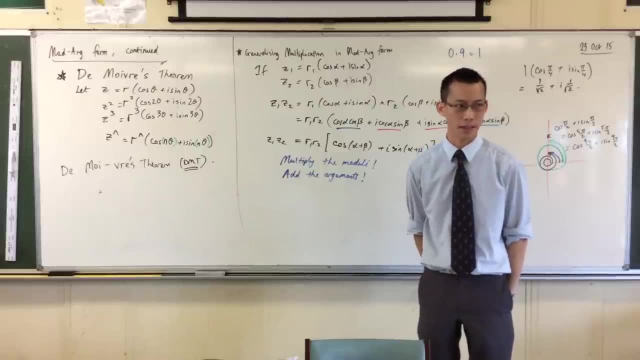 De Moivre's theorem. This is a very special case. Because it's special, It does come up repeatedly, In fact, you'll see it appear in exercise 1.2.. You can take quite significant advantage of it. okay, Now, before I let you loose, just to finish working, okay. 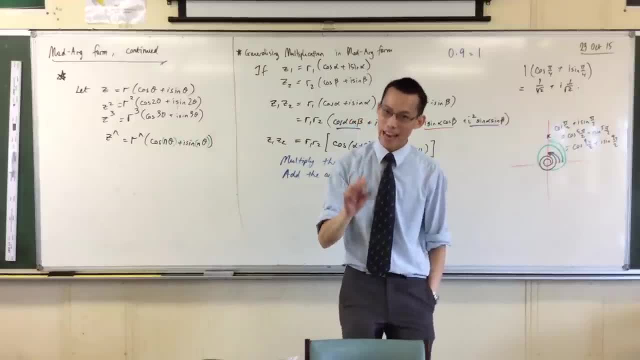 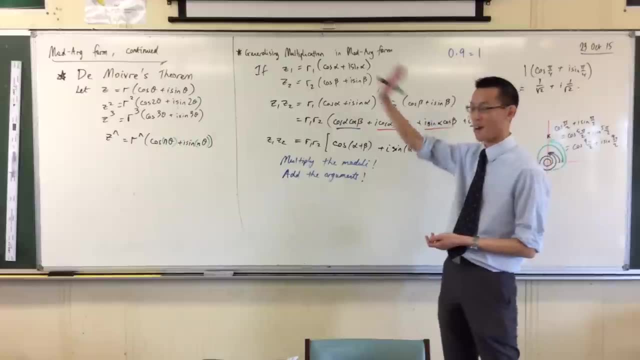 And I'm going to write it first and then I'm going to teach you how to pronounce it. Okay, So here is the theorem Now. I have heard like a hundred different pronunciations of this name. okay, Let me teach you first, like the pieces, before we do this thing. okay, 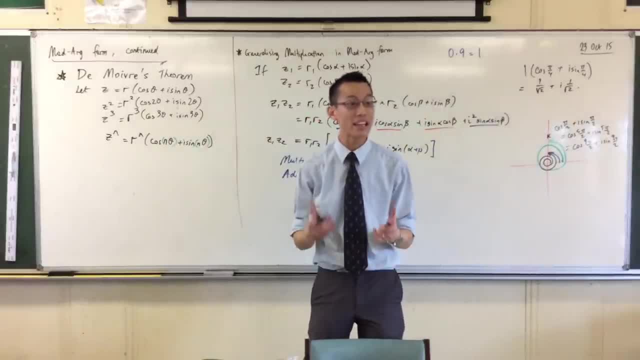 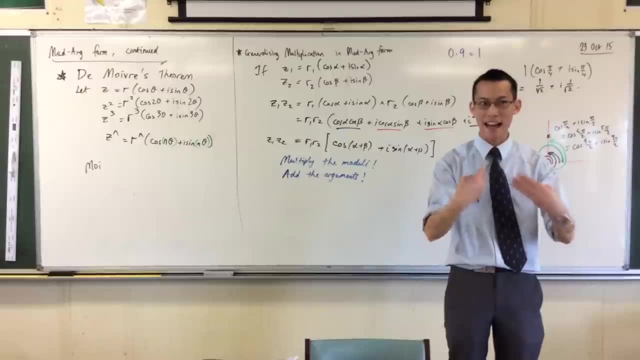 Firstly, remember, it's French, It's French, right, It's French. So, in French, when you see this word, what do you say? You say moi, right, As in you know me, okay. You do not say moi okay. 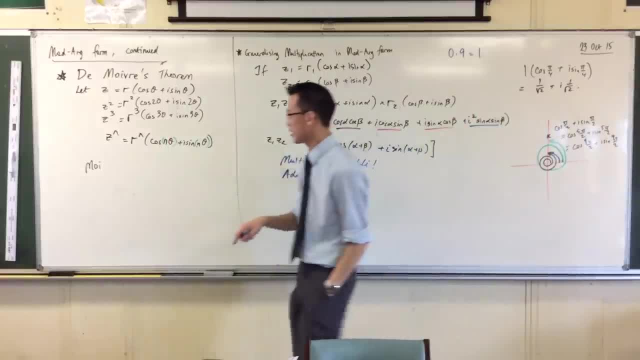 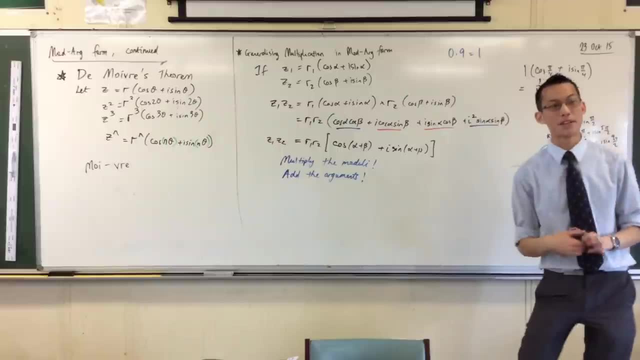 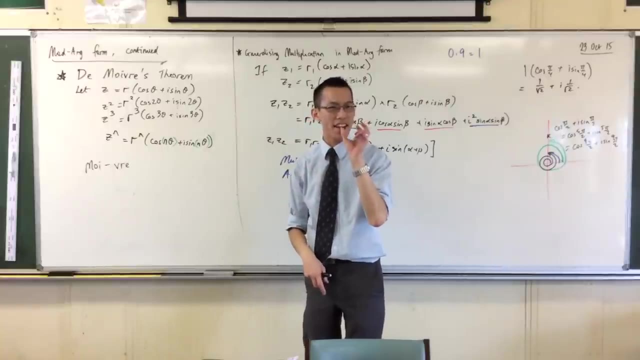 Don't say moi Now. secondly, when you see this, okay, Now you might know. there's a famous art gallery which has this as the end of its name as well. Okay, It's this R here, right, It's not quite like we say R. 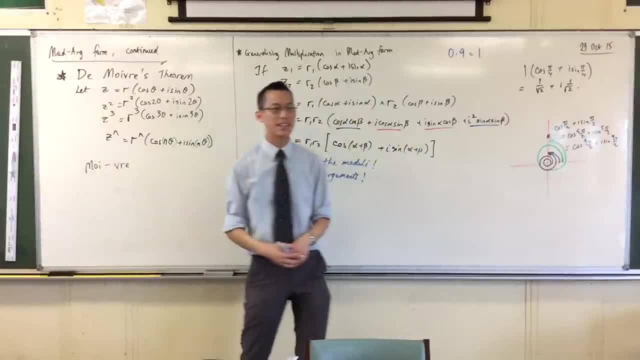 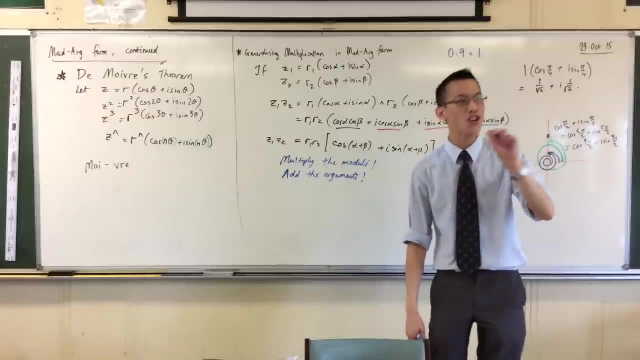 There's no vowel in here, okay. So the way you would say this is: as It's not like There's no hard R sound on the end, It's just, You almost don't hear it. okay, You almost don't hear it. 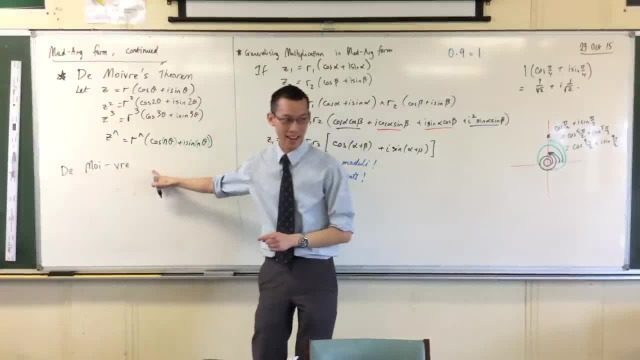 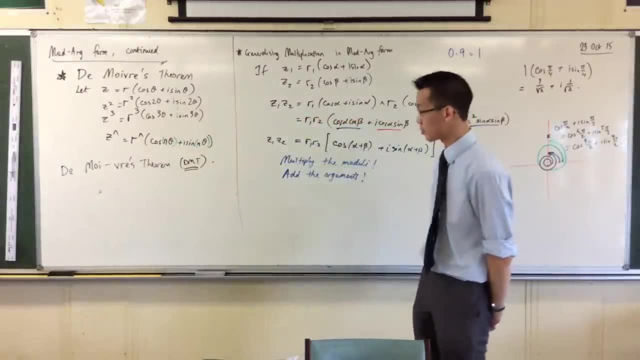 This is de Moire's theorem. okay, De Moire's theorem, This is a very special case. Because it's special, it does come up repeatedly. You'll see it appear in exercise 1.2.. You can take quite significant advantage of it, okay. 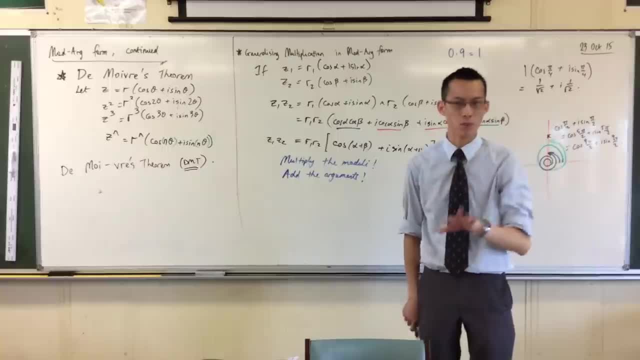 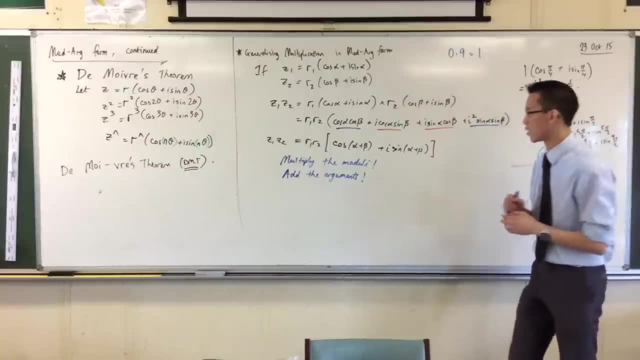 Now, before I let you loose, just to finish working, okay, I wonder, based on all this generalizing we have done, okay, I wonder what you would make of you. remember how I said: okay, What happens when we do repeated multiplication by i? okay, 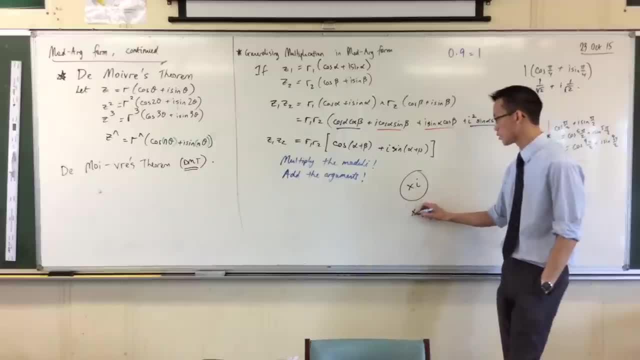 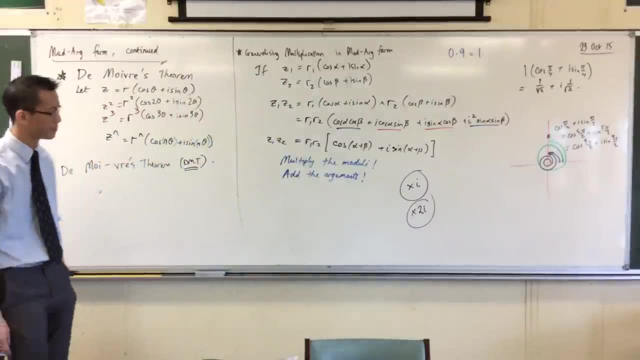 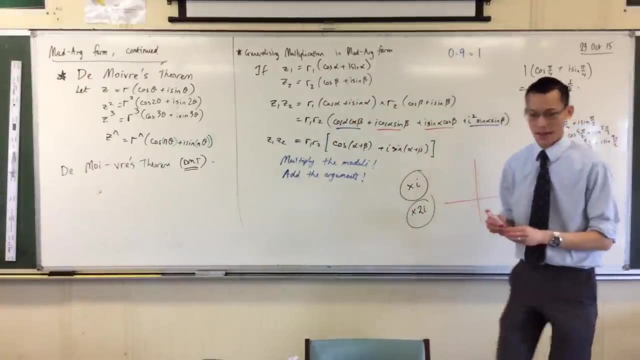 What do you think would happen if I did repeated multiplication by something like 2i? Don't shout it out, Just try and picture what might be happening. Now, to guide you before I just draw it for you, okay, To guide you, let me remind you where is 2i on our complex plane. 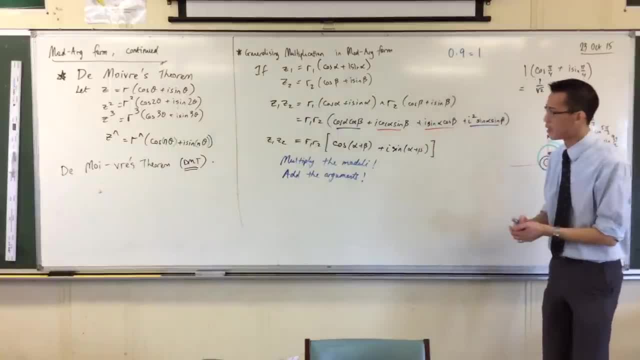 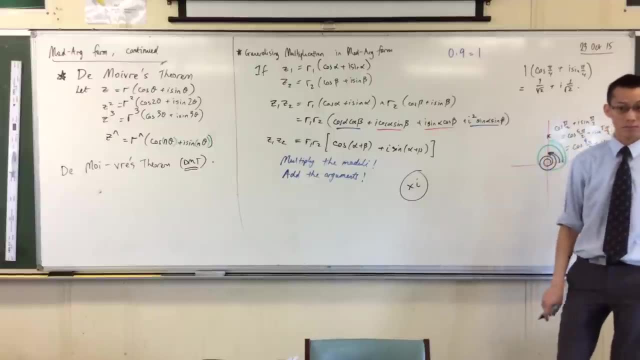 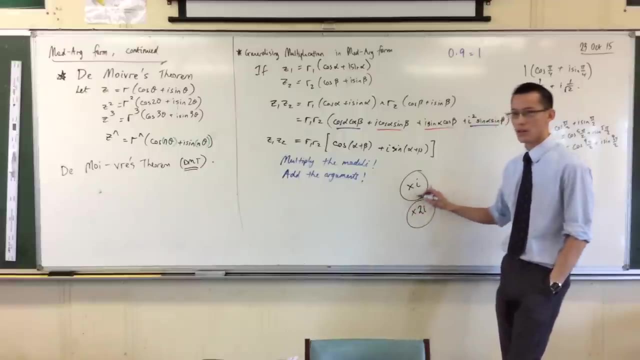 I wonder, based on all this generalizing we have done okay, I wonder what you would make of you remember how I said: okay, What happens when we do repeated multiplication by i? okay, What do you think would happen if I did repeated multiplication by something like 2i? 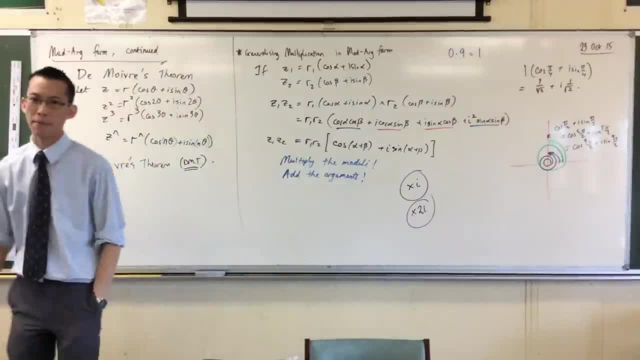 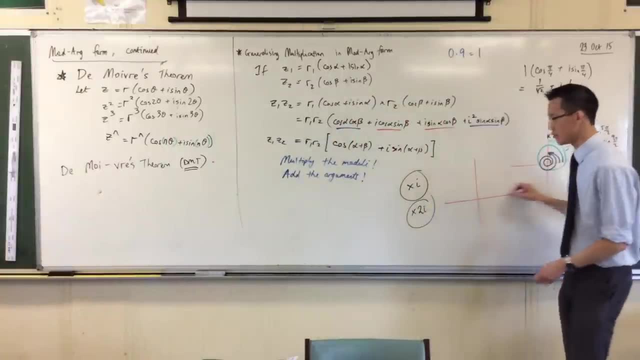 Don't shout it out, Just try and picture what might be happening. Hmm, Now to guide you. before I just draw it for you, okay, To guide you, let me remind you where is 2i on our complex plane. 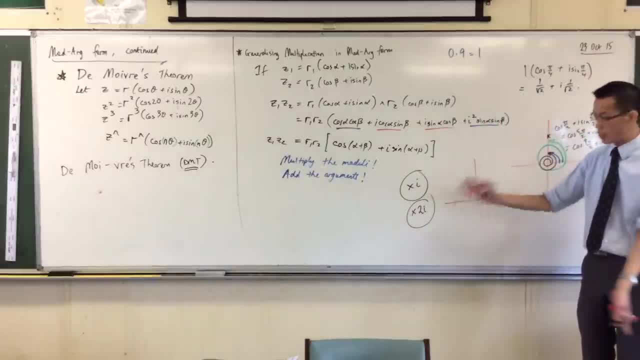 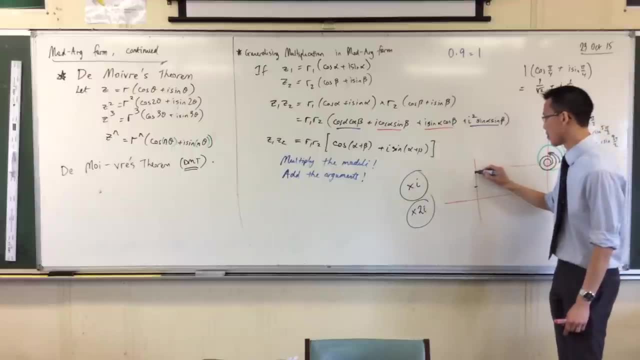 It's still on the imaginary axis, There's no real part to it, okay. But if i is here, then 2i is twice as far away. It's up here, There's 2i, okay. So I hope you can see now. 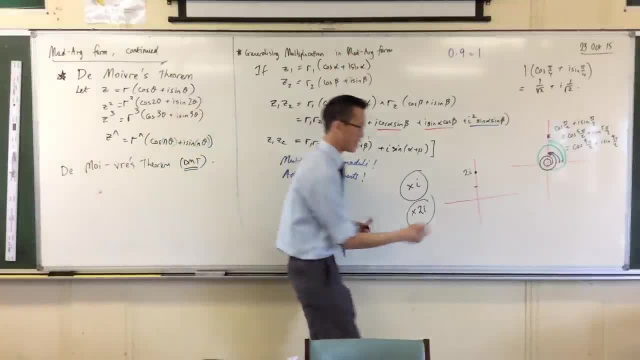 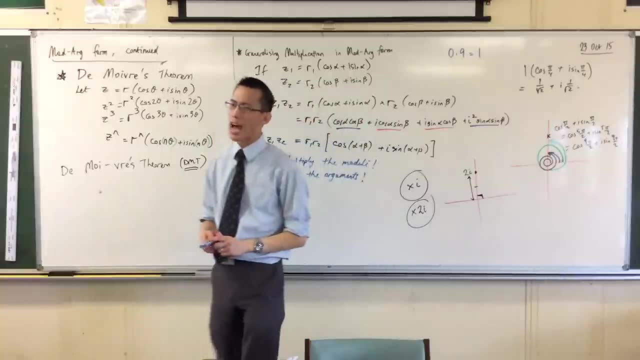 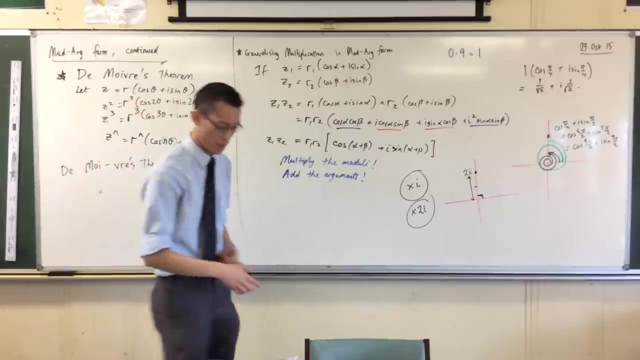 To get this in mod-arg form. you can see what the argument is and you can see what the modulus is. okay, So now what would you predict would happen when you multiply by 2i repeatedly? Are you ready for the picture? 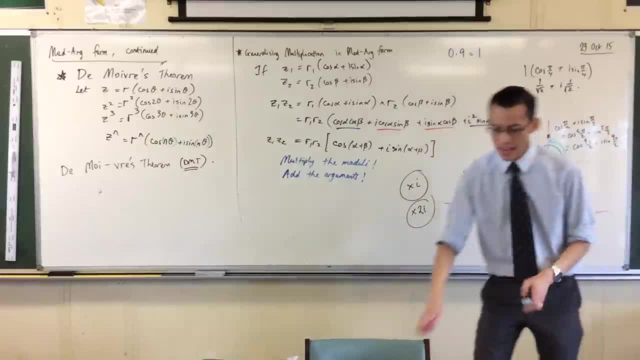 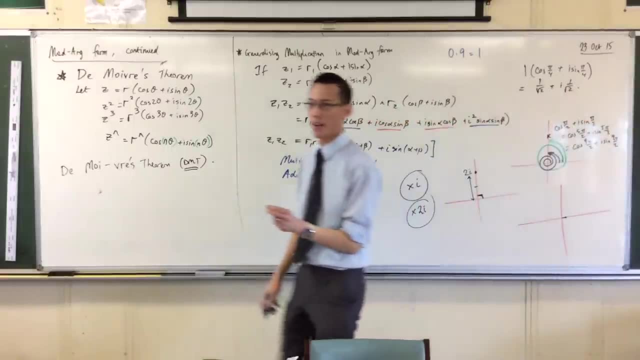 Just think about it. I'm going to start nice and small. okay, If I plot 1 and I plot it like there, I need to start small, and I hope you can see why. okay, Well, the first multiplication by 2i, that's easy. 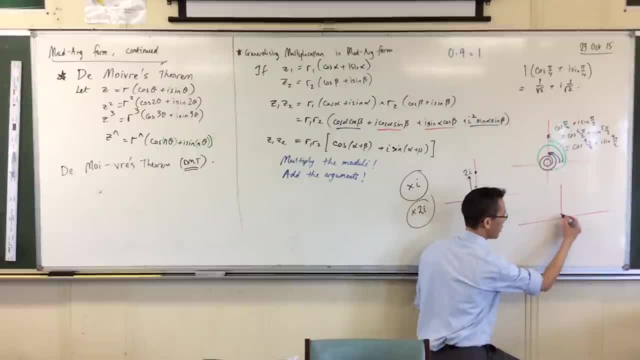 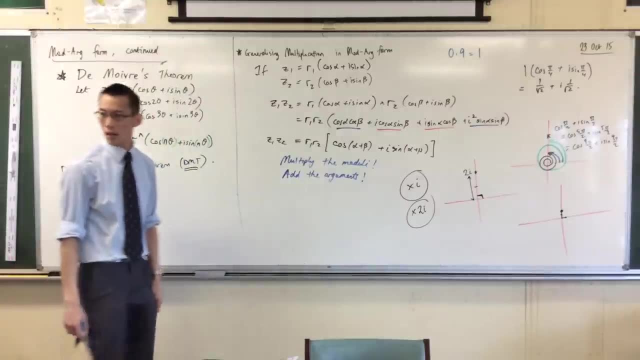 I've already shown you where that is okay. So if that's 1,, then 1,, 2, there will be 2i. You see that There's my first multiplication. What will happen for the next one? Okay, firstly, I'm going to rotate back onto the real axis, right? 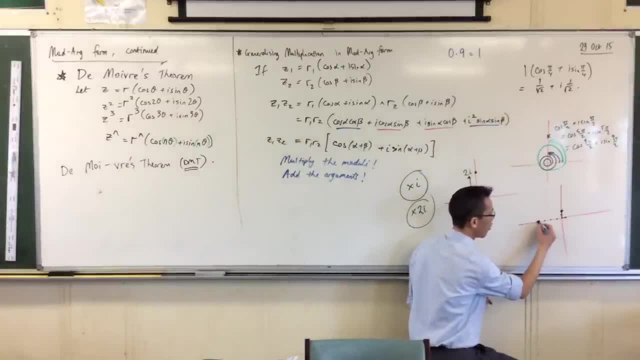 But I'm going to be 1,, 2,, 3,, 4,, twice as far away. You see that What happens when I do my third multiplication? I'm going to be 1,, 2,, 3,, 4,, 5,, 6,, 7.. 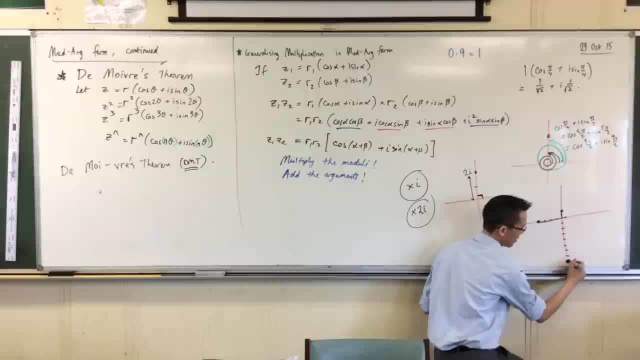 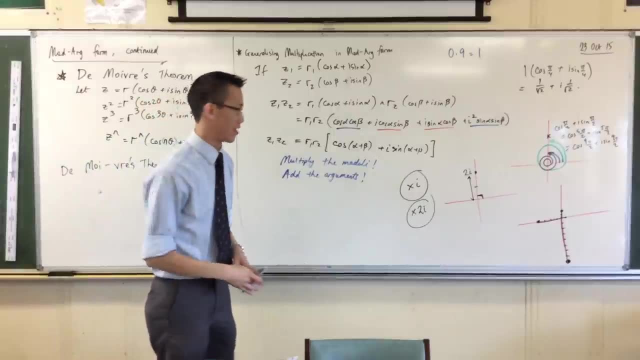 1, 2,, 3, 4,, 5,, 6,, 7,, 8.. And I've rotated around another pi on two radians. okay, If I multiplied one more time. okay, Because it's 2i, then 2i to the power of 4, of course. 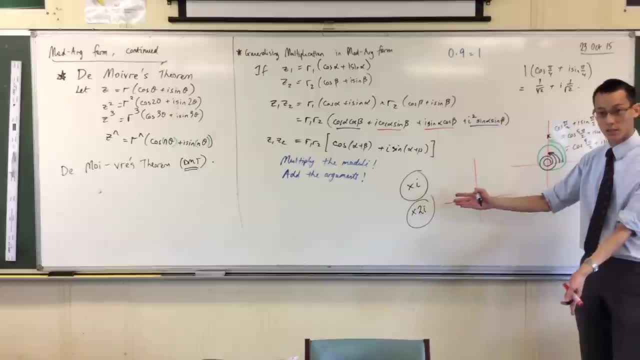 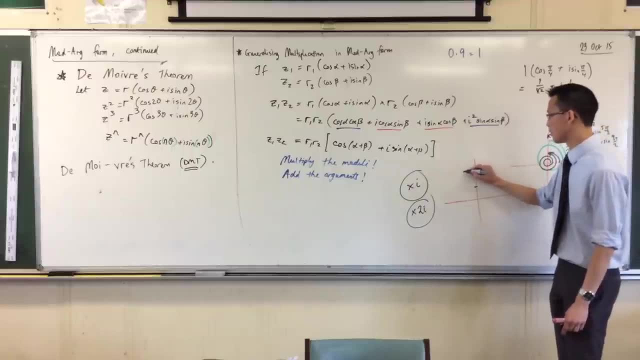 It's still on the imaginary axis, There's no real part to it, okay. But if i is here, then 2i is twice as far away. It's up here, There's 2i, okay. So I hope you can see now to get this in mod-arg form. 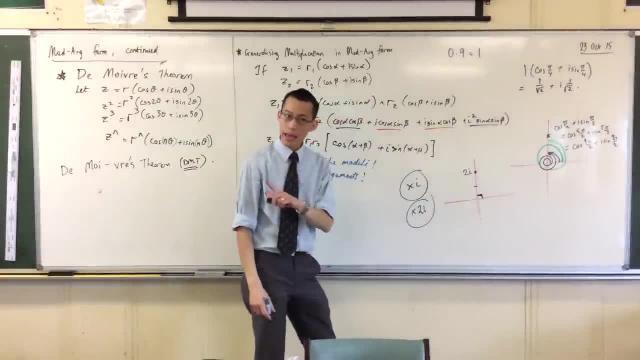 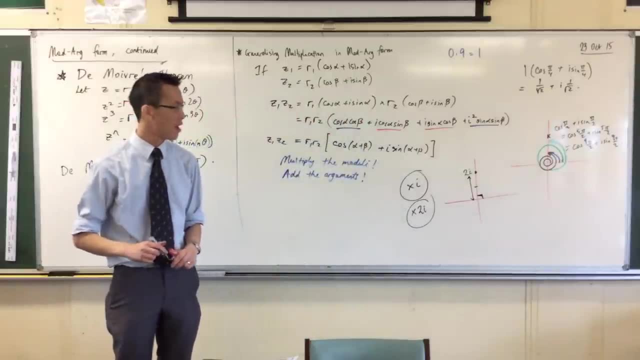 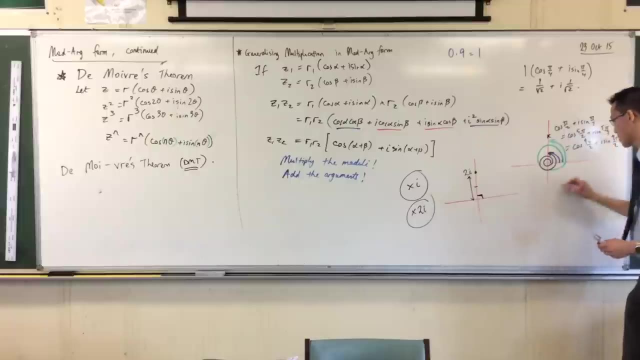 you can see what the argument is and you can see what the modulus is. okay, So now, what would you predict would happen when you multiply by 2i repeatedly? Are you ready for the picture? Just think about it. I'm going to start nicely small, okay. 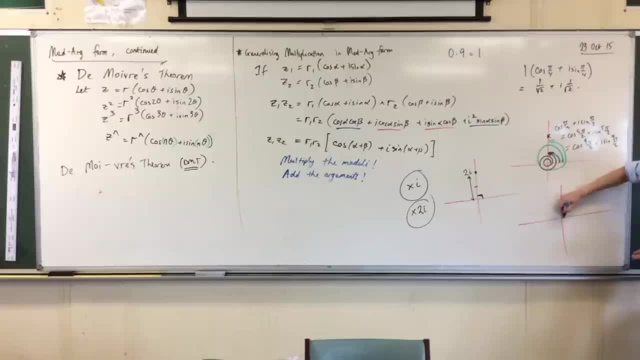 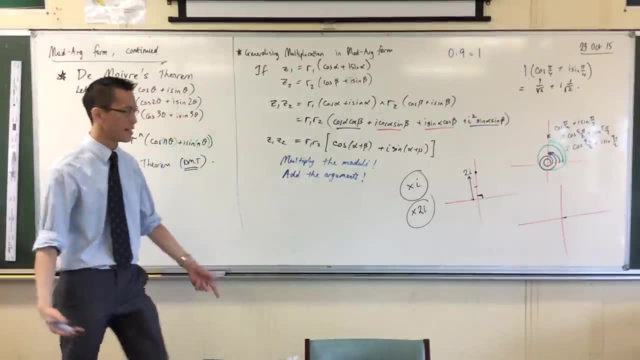 If I plot 1, and I plot it like there, I need to start small, and I hope you can see why. okay, Well, the first multiplication by 2i, that's easy. I've already shown you where that is okay. 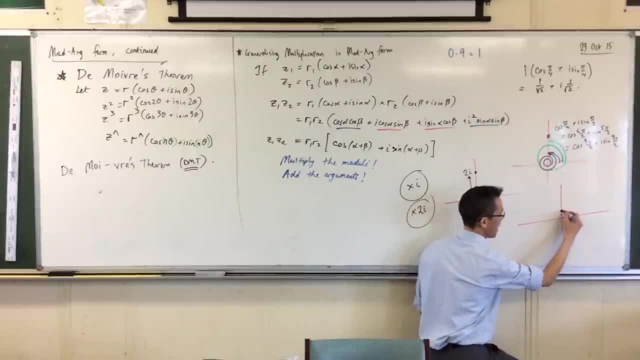 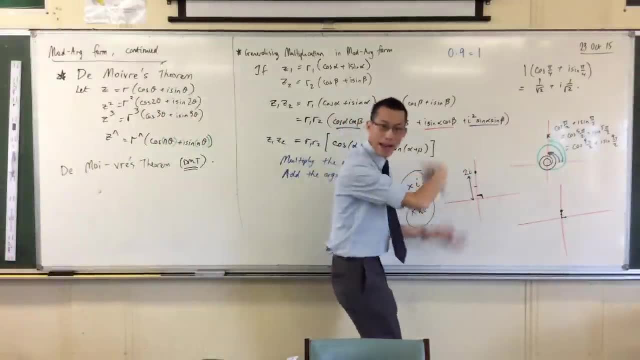 So if that's 1, then 1,, 2, there will be 2i. You see that There's my first multiplication. What will happen for the next one? Okay, firstly, I'm going to rotate back onto the real axis, right? 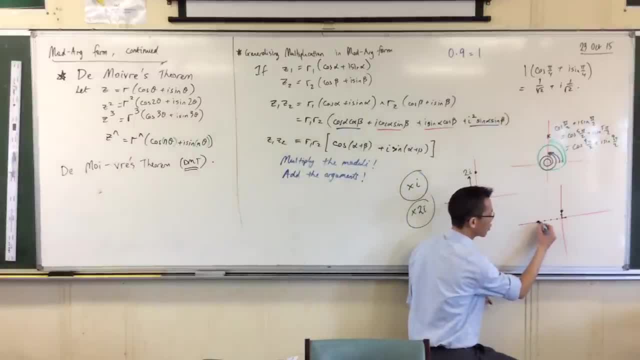 But I'm going to be 1,, 2,, 3,, 4,, twice as far away. You see that What happens when I do my third multiplication? I'm going to be 1,, 2,, 3,, 4,, 5,, 6,, 7,, 8.. 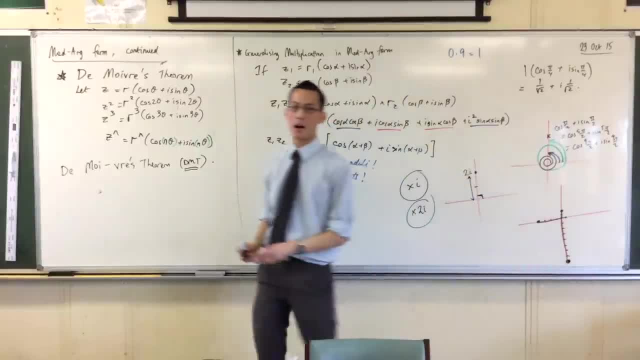 And I've rotated around another pi on two radians. okay, If I multiplied one more time. okay, Because it's 2i. then 2i to the power of 4, of course is 2 to the 4 times i to the 4.. 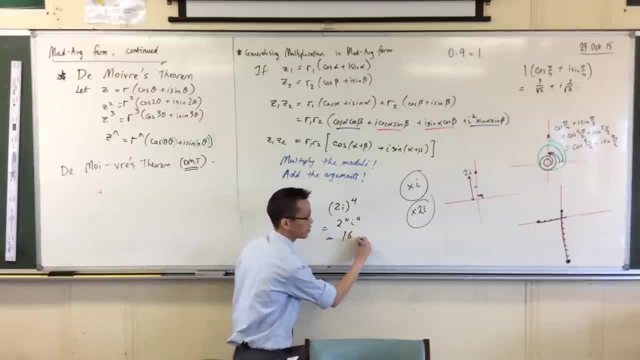 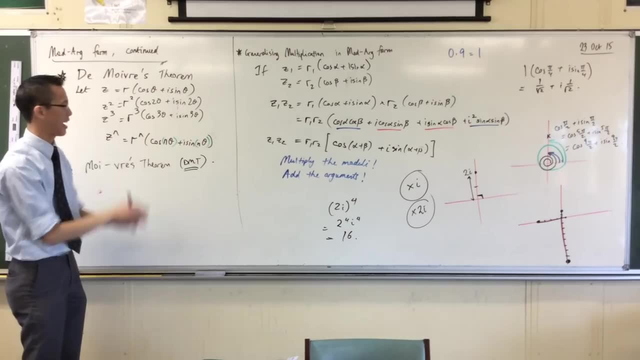 But you know what i to the 4 is? It's 1. So it's just 16 back on the real axis. okay, So get a sense by the geometry of these numbers. okay, These are very powerful results, but you need to see them. 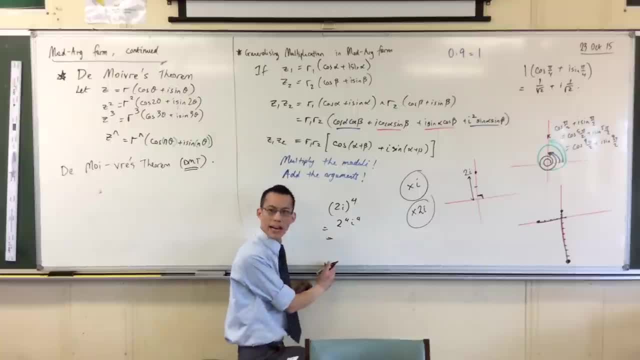 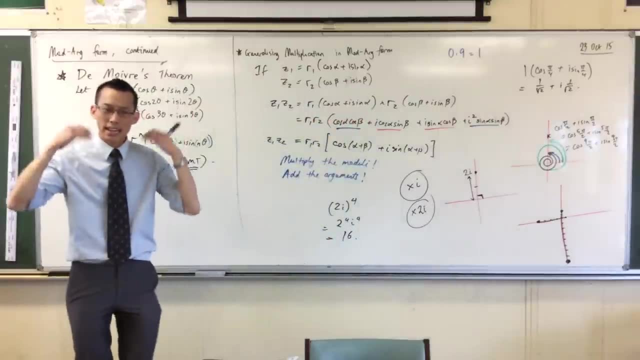 is 2 to the 4 times i to the 4.. But you know what i to the 4 is, It's 1.. So it's just 16 back on the real axis, okay, So get a sense by the geometry of these numbers. 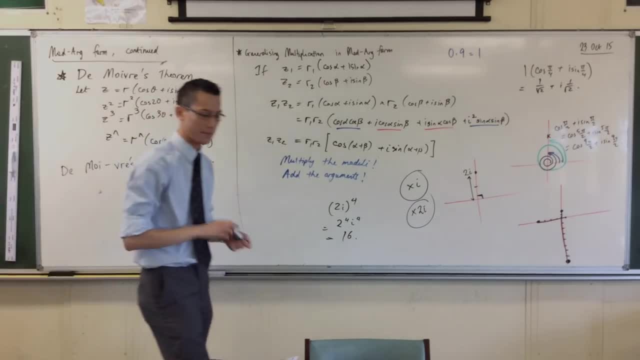 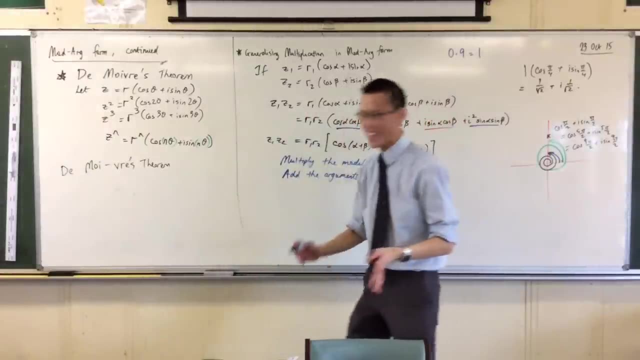 Okay, These are very powerful results, but you need to see them Now. if you're like, if you're like I've tried and I've tried and I've tried and I still sound like an idiot, then just call it that, okay. 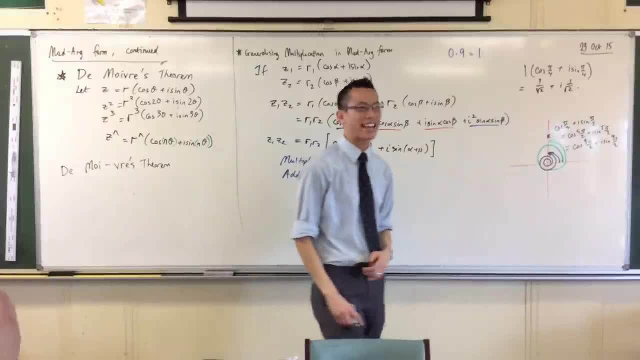 Now, if you're like I've tried, and I've tried, and I've tried and I still sound like an idiot, then just call it that. okay, Save yourself some trouble. Let me tell you: Well, see the French guy. 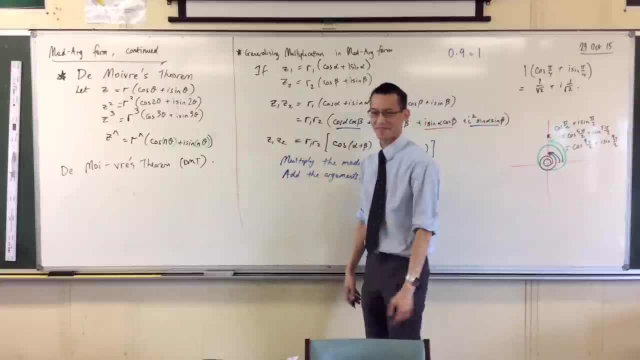 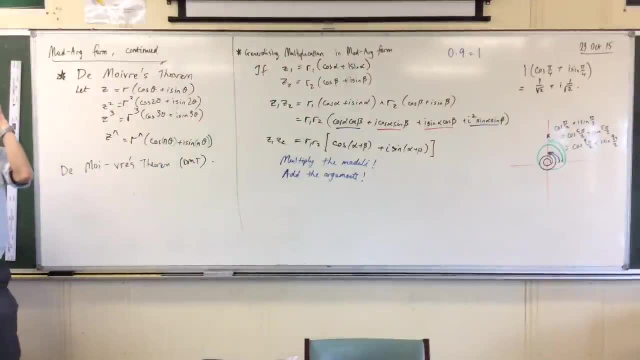 Argand or de Moivre. No, for Argand we can say Argand. Okay. now please don't, Please don't, as I've heard many well-meaning people say. don't pronounce this as Moivre. 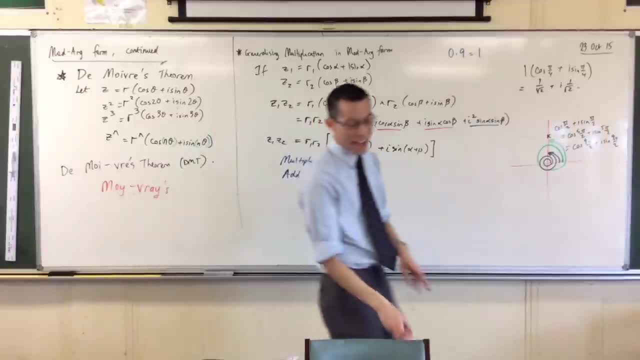 Moivre. Okay, Now, Moivre. Now I've heard people say it's- And, by the way, they say it with great authority, like this is how it's- And they say, yeah, yeah, I know that. 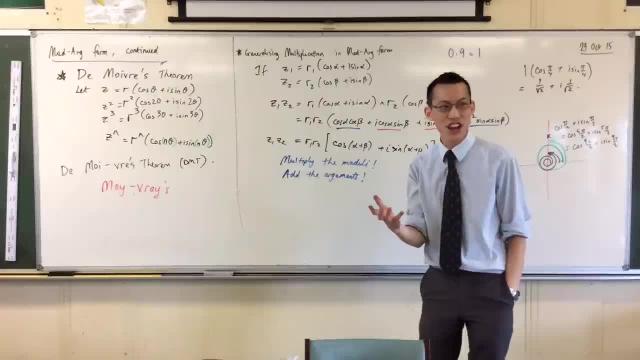 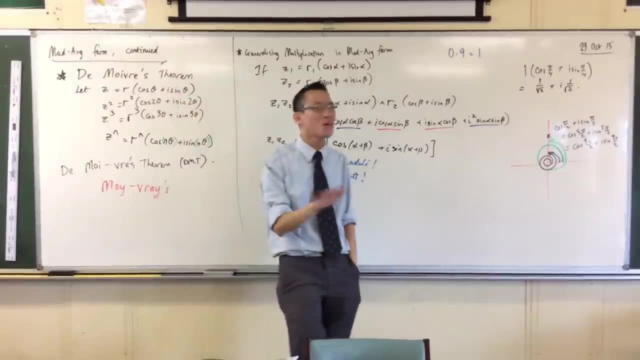 It's de Moivre's theorem. right Now, it's French, It's not Spanish. okay, It's not like: oh yeah, oh yeah, there's Chile and then there's de Moivre, right, No, no, no, okay. 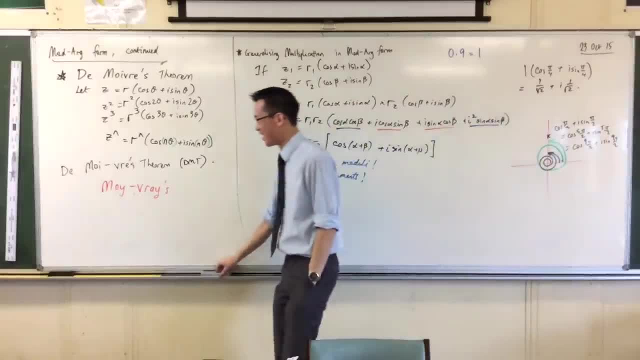 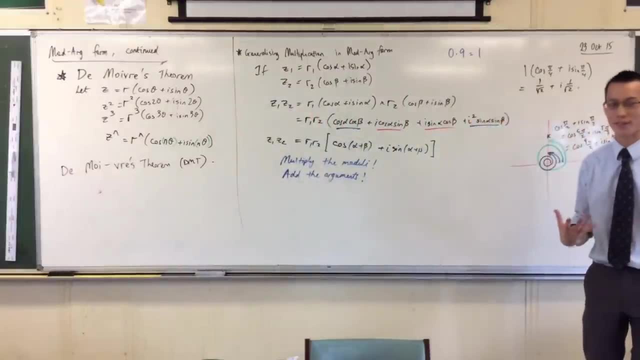 Not Spanish, It's French okay. So So, no, Moivre, okay, Compadre Moivre, it's not Spanish De Moivre. 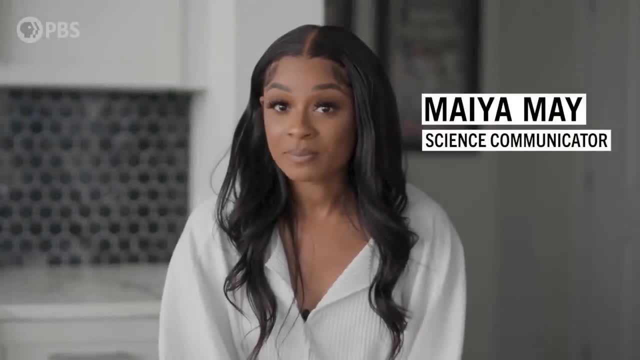 Is one degree of warming really that big of a deal? How about two? Could one and a half or two degrees of warming from pre-industrial levels mean doomsday or game over? Seems kind of extreme, but we know that the earth will look different as the climate warms because we can already see some of it happening around us. And there are some pretty amazing models that predict what the world would look like with changes set in motion by just a bit more warming. So who's going to be 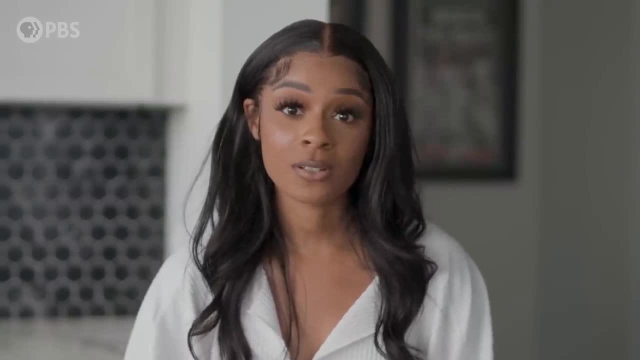 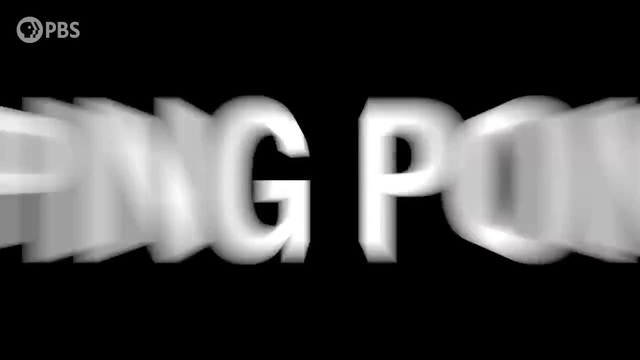 affected? Where will we feel the effects first? And how can such a small change matter in such a big way? The answer lies in understanding tipping points. But when will we reach them? 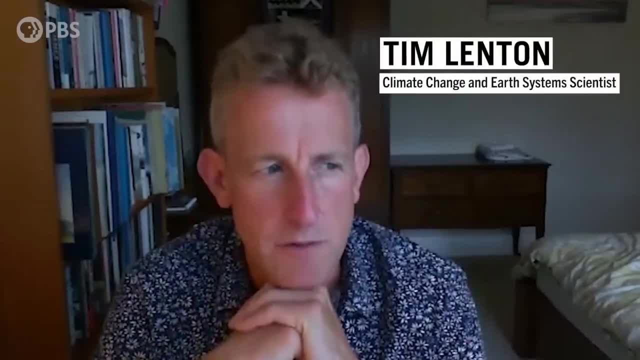 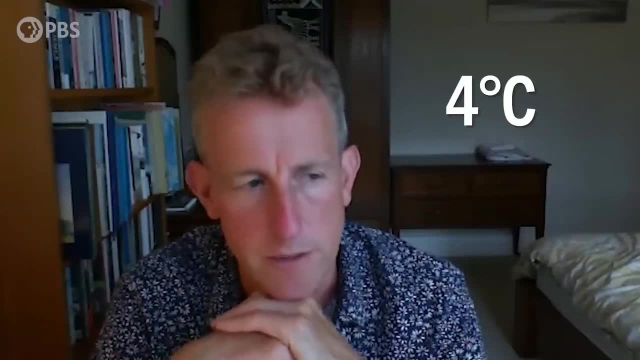 In the early 2000s, the kind of general consensus would have been maybe we're at risk of tipping points at, say, four degrees C of global warming, where now we're just publishing a study which essentially says it's seeding. 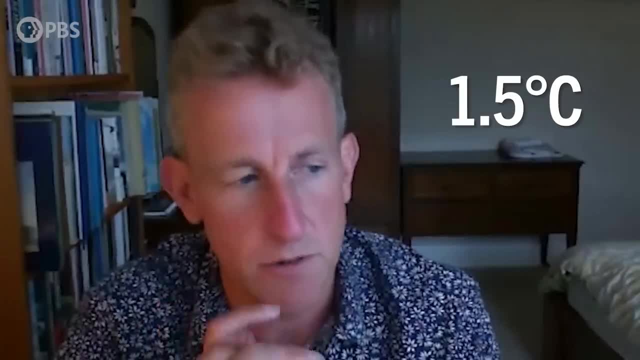 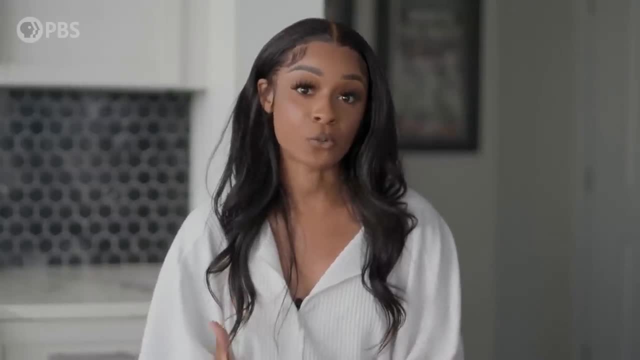 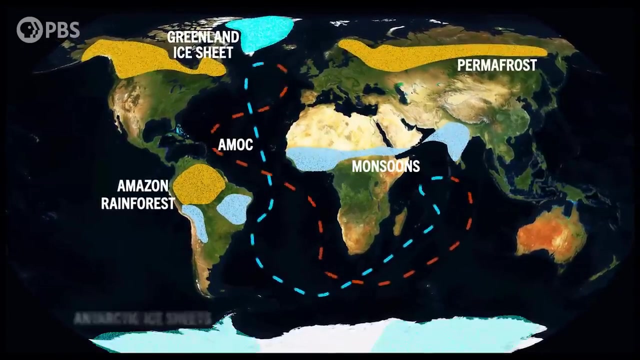 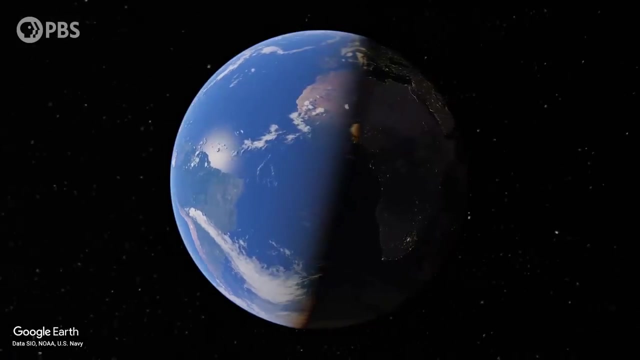 And that's very close to our current level of about 1.1 degrees of warming. So let's find out what the world would look like if we hit six of the 15 most pressing tipping points identified by the International Panel on Climate Change. First, we'll explain how changes that could be set in motion very soon would fundamentally change our world. And stay with us until the end when we 're back.